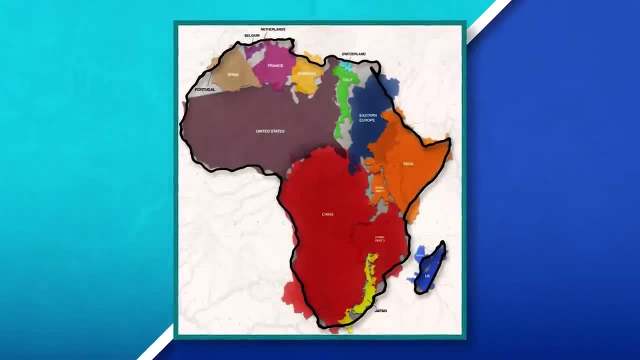 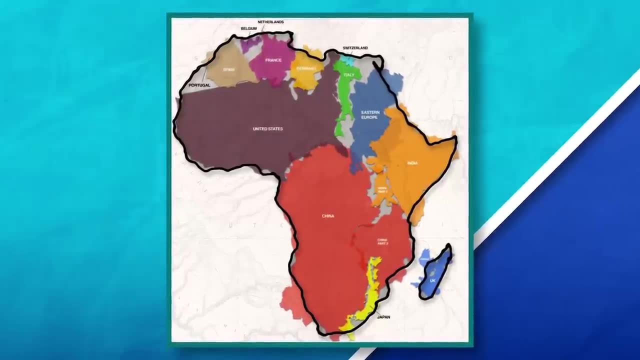 States, Italy, Germany, France, the Netherlands, Belgium, Spain, Portugal, almost all of Eastern Europe, India, China, Japan and the United Kingdom, all inside Africa. But you would never know that if you just went off the Mercator map, If we were to put all these circles around the globe and then 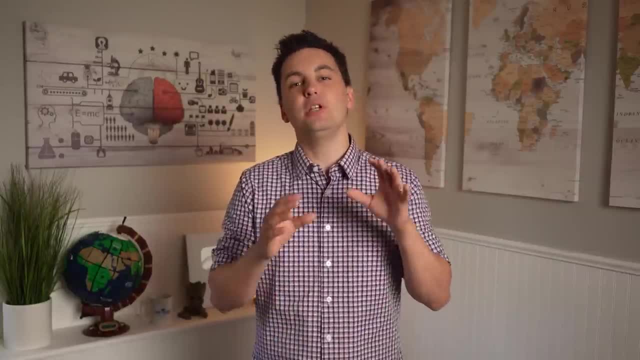 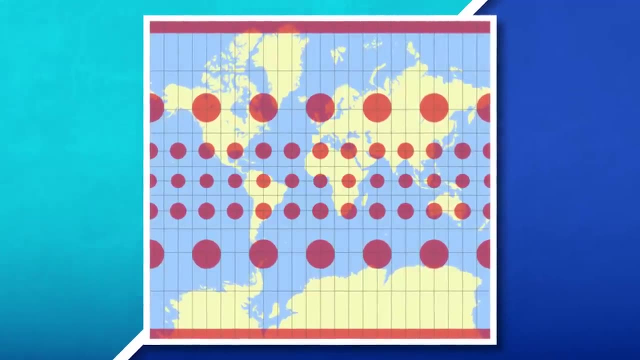 project them onto the Mercator map. we would never know that if we just went off the Mercator map. If we went off the Mercator map projection, we would get an image that looks like this: Notice how the circles still keep their shape, but the size varies depending on the location of 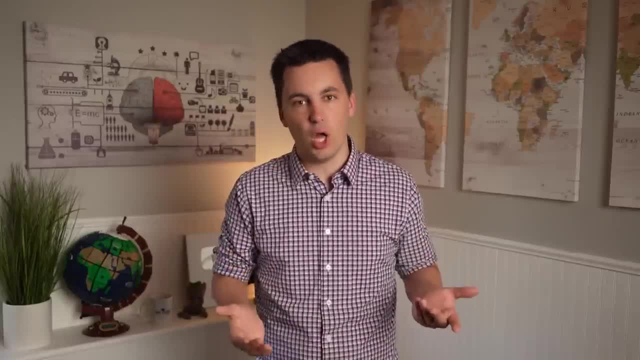 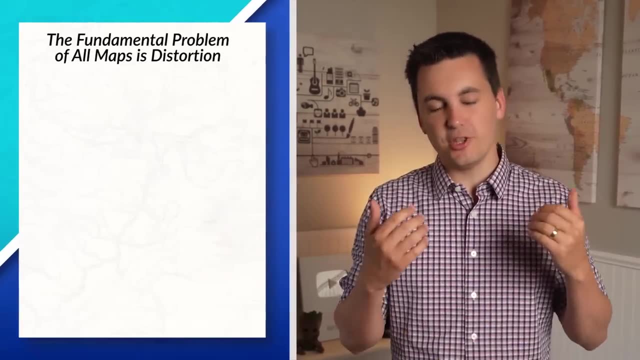 the circle. And it isn't just this map that has some pretty major flaws. In fact, every map you have ever looked at has distortion. Whenever we try to view the globe on a flat surface, we can see that distortion impacts either the direction, the shape, the area, distance. 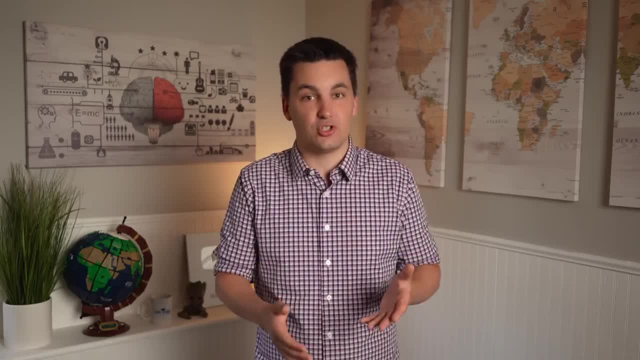 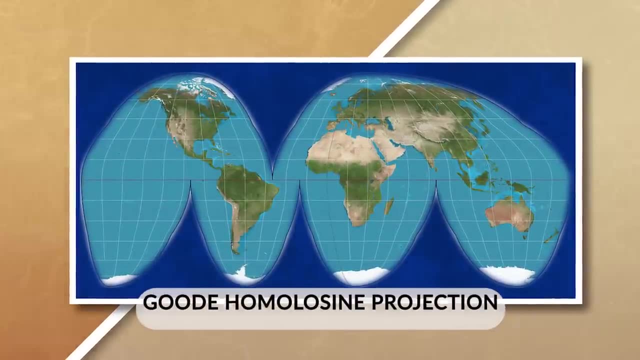 or sometimes all of them at once. Okay, so if the Mercator map projection is flawed, then what map projection should we use? Well, we could use the Good-Homelsene projection, which is an interrupted map. This map projection is an equal area projection. It excels at showing. 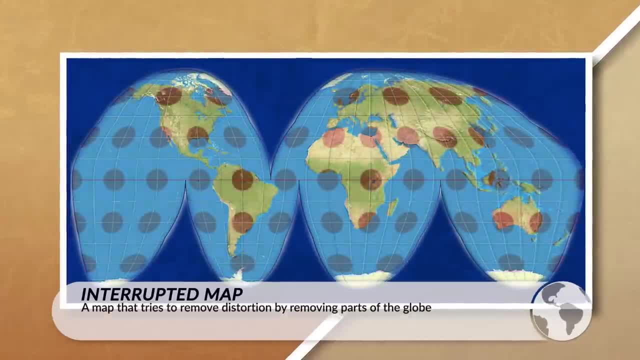 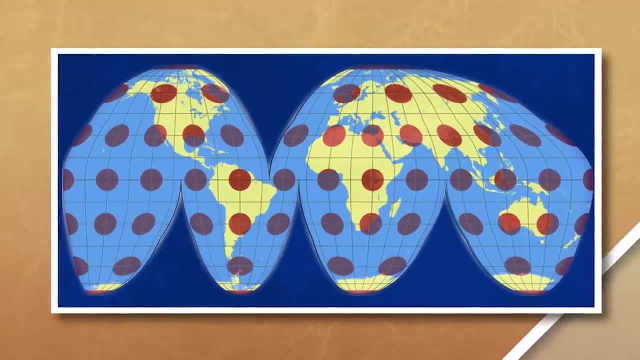 the true size and shape of the Earth's land masses, but has distortion with distance and distortion near the edges of the map. This map is also not that helpful for direction, since it is an interrupted map. Another interrupted map that we could use is the Fuller. 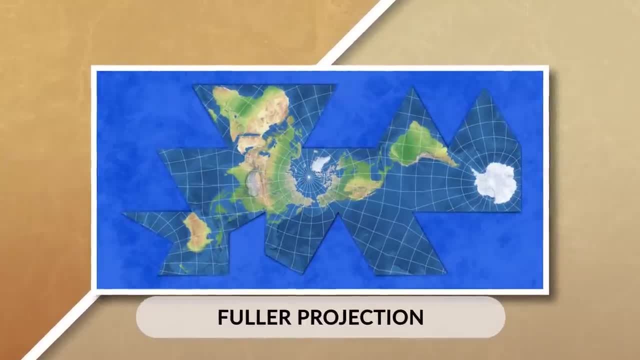 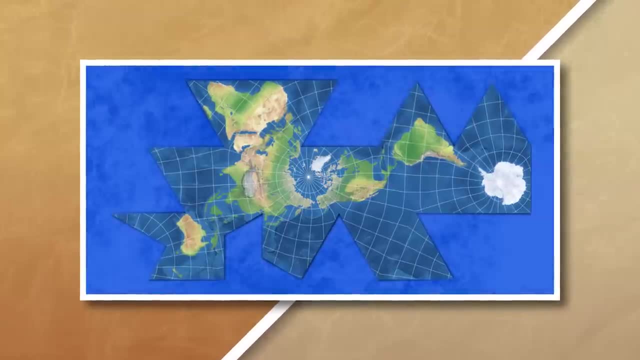 map projection. This projection shows land masses without an eruption and maintains accurate size and shape. It does not use the cardinal directions, which makes it kind of difficult for people to read. Plus, it still struggles with the distortion, especially as you get farther away from the 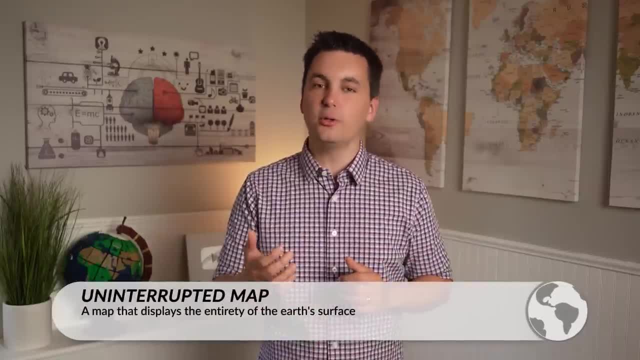 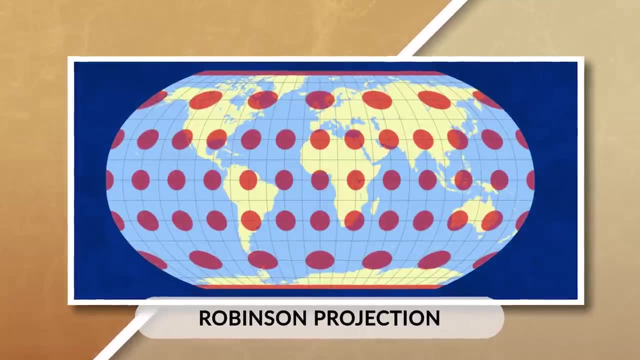 center point. If we go back to map projections that are uninterrupted, we could look at the Robinson projection. This map projection puts the majority of the distortion at the poles and it maintains the true size and shape of the land masses. We could also look at the Winkle. 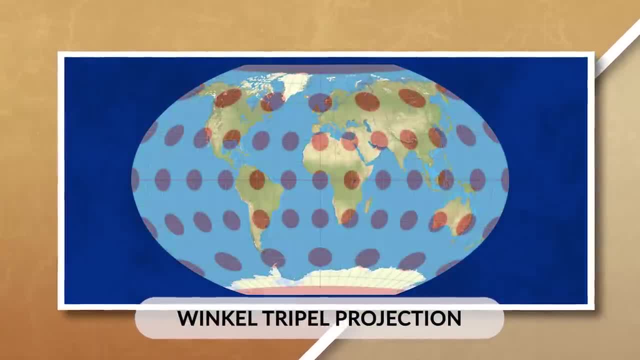 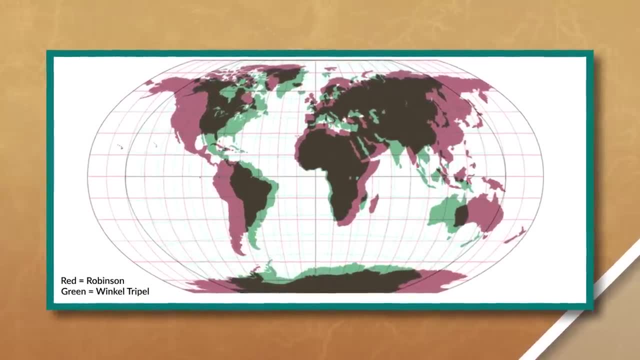 triple projection, which is similar to the Robinson projection. This projection is rounder in shape and also larger. This map projection is also not that helpful for direction, since it is not that accurate. This map projection is similar to the Robinson in that it spreads distortion. 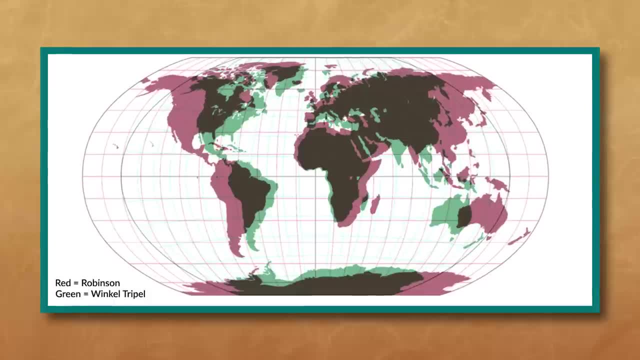 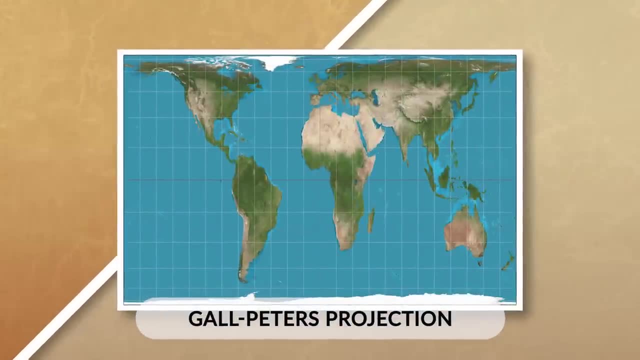 out throughout the entire map but tries to concentrate as much of the distortion as possible at the poles. There's also the Gauls-Peter projection, which is one of the most accurate map projections at showing the true size of land masses. But we can see immediately that it. 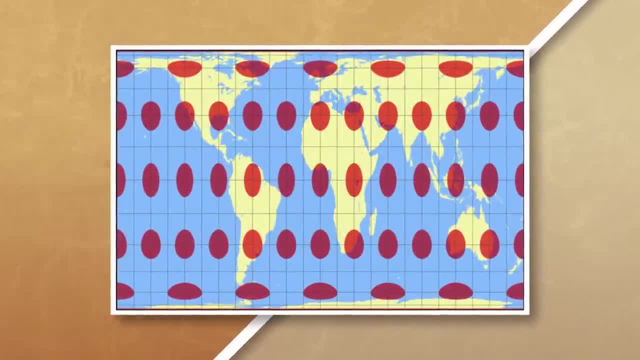 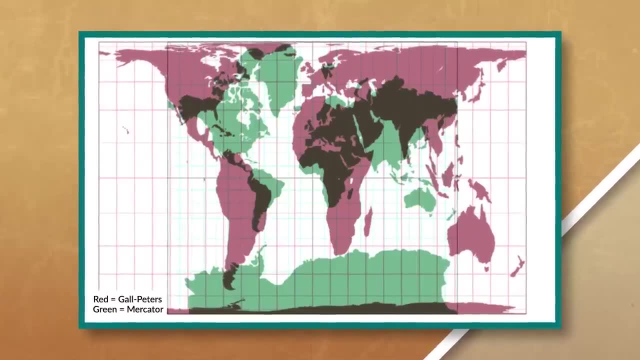 has a significant amount of distortion in the shape of the land masses and also direction. Oftentimes people will compare the Gauls-Peter projection with the Mercator map projection. Here you can easily see the difference between the Gauls-Peter projection and the Mercator map projection. Here you can easily see the 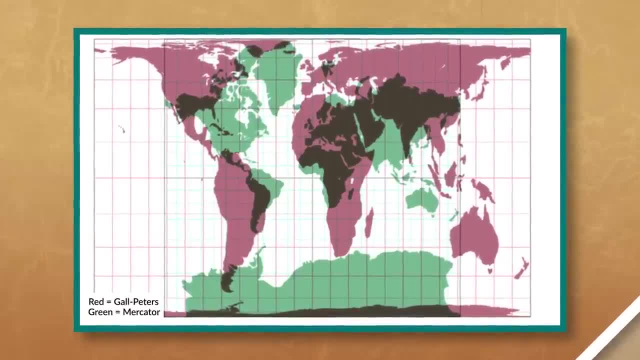 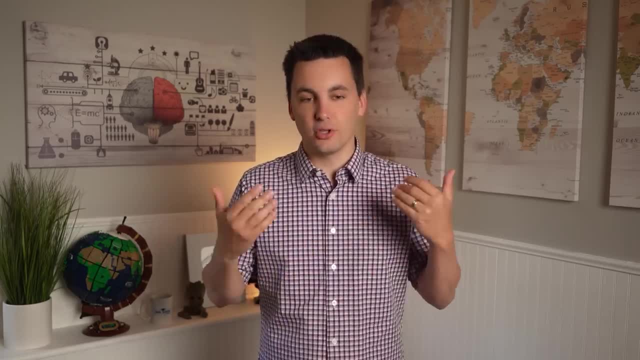 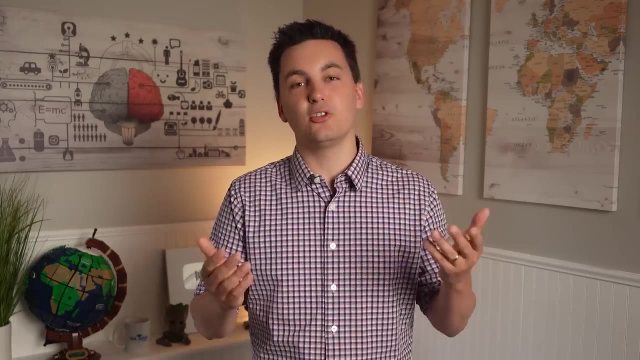 difference in the size, location and shape of the land masses. Honestly, we could go on and on with map projections. There are hundreds of different map projections that all depict the globe in a different way. Each map projection is better suited for different purposes and each projection is impacted by distortion in different ways. 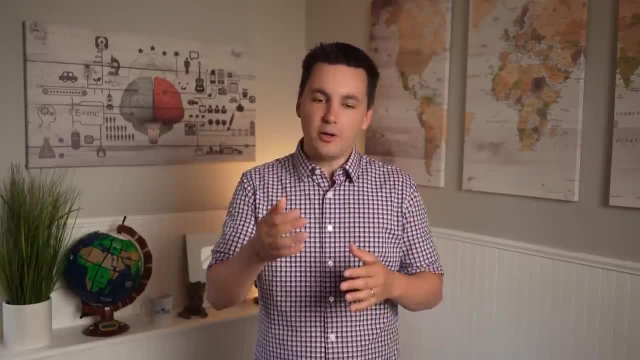 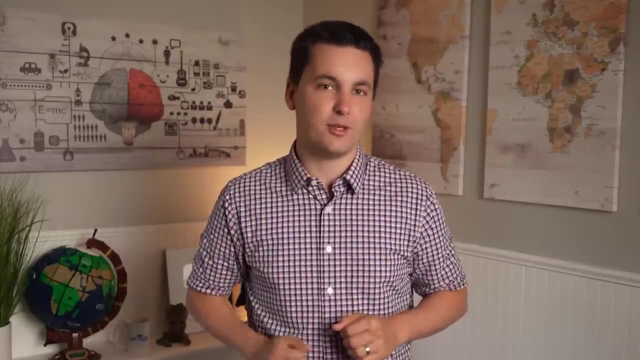 Now, people use maps for a variety of different reasons, but regardless of the use, we can generally categorize maps into two main categories: reference maps and also thematic maps. Reference maps are informational maps. These maps would be used to find the boundaries of a place. 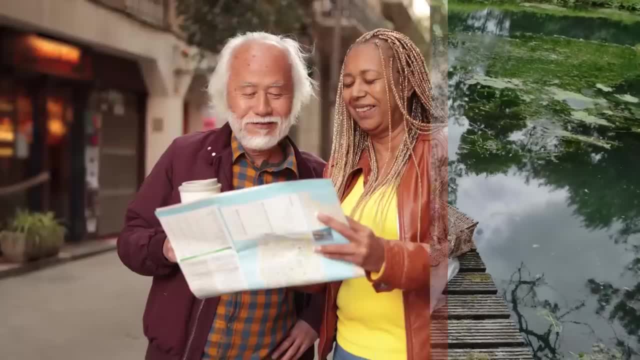 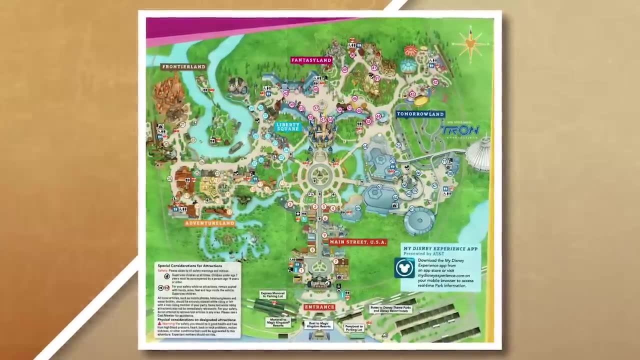 look at different geographic features or be able to be used to get directions from point A to point B. For example, if you go to Disney World, you'll probably use a reference map to move around the park, Or if you're going to be going on a hike with friends, you'll use a topographic map. 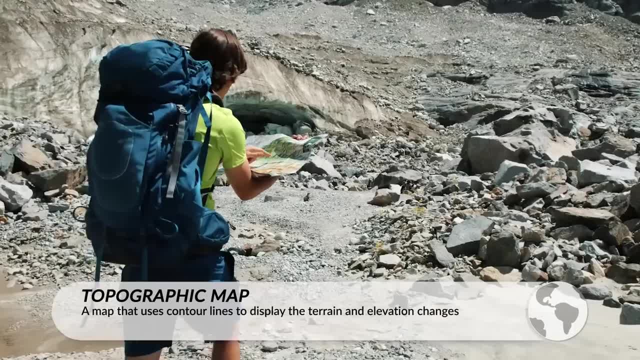 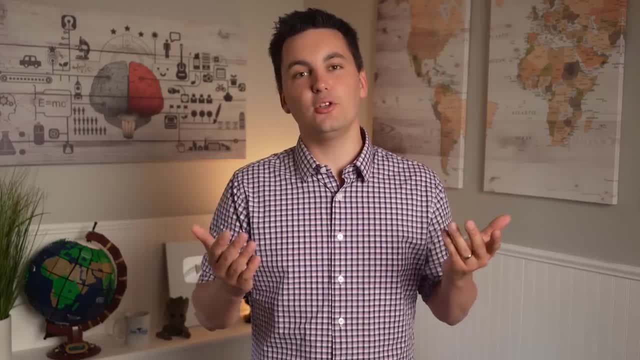 to understand how the elevation will change on your hike. Or let's say you're ready for some dinner and you're trying to get to the nearest Chipotle, You'll want to use a reference map for directions. Or maybe you want to use a reference map to better understand the public transportation. 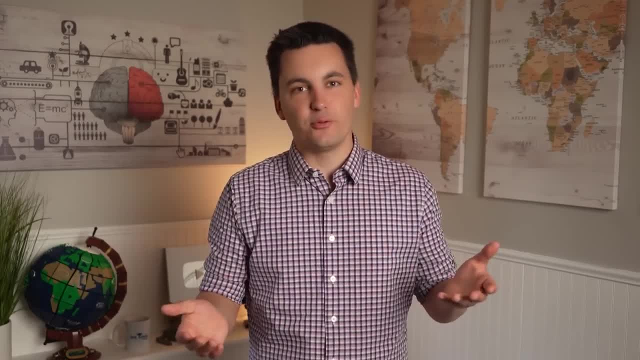 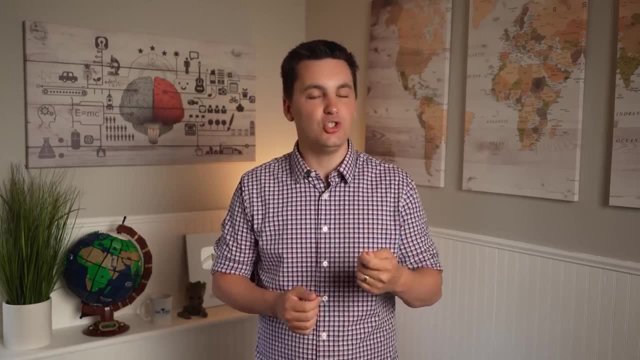 in an area. All of these are examples of reference maps. Now, when using reference maps, you'll often be looking at absolute and relative distance, which can sometimes be confused with absolute and relative location or direction. Many students mix these terms up, so it's important to remember. 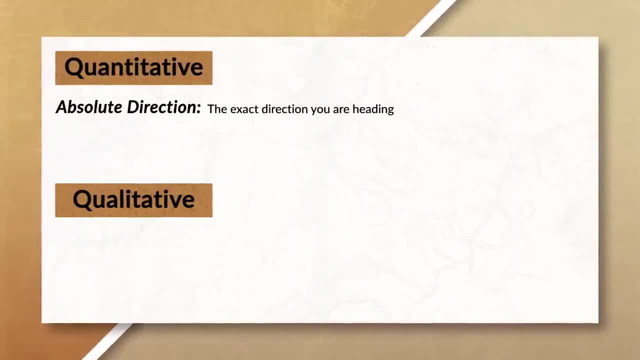 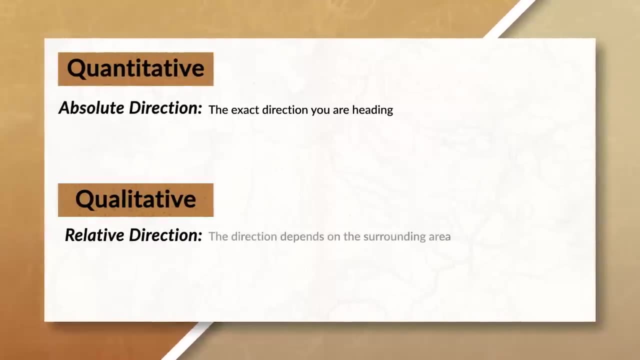 the difference between them. Absolute direction is the exact direction you are heading. For example, if you were traveling east of your current location, your compass will show 90 degrees. Relative direction is when you use the map to find a particular location or direction. So if you're 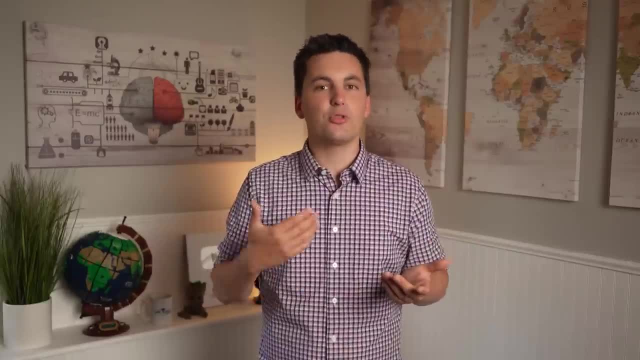 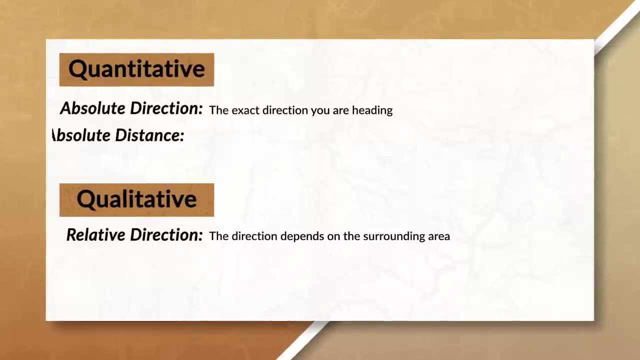 heading north of your current location, you'll want to use the surrounding area for direction. For example, I'm north of you right now. Notice, the direction depends on the current situation. It's not precise and could change. Absolute distance is the exact distance between two. 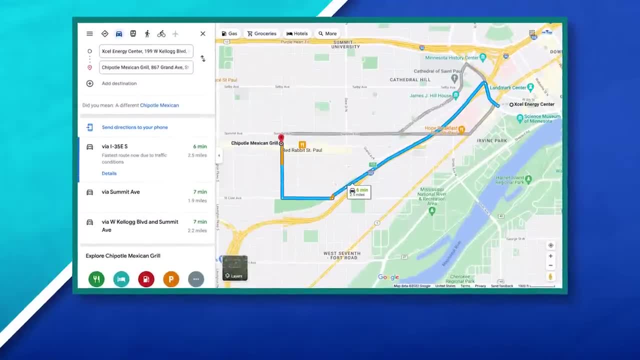 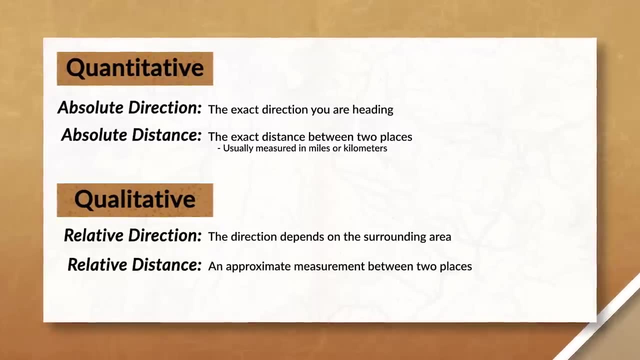 places usually measured in miles or kilometers. For example, Chipotle is 2.5 miles away from the Xcel Energy Center. Relative distance is an approximate measurement between two places usually talked about in time or direction. For example, Chipotle is about 6 minutes away from. 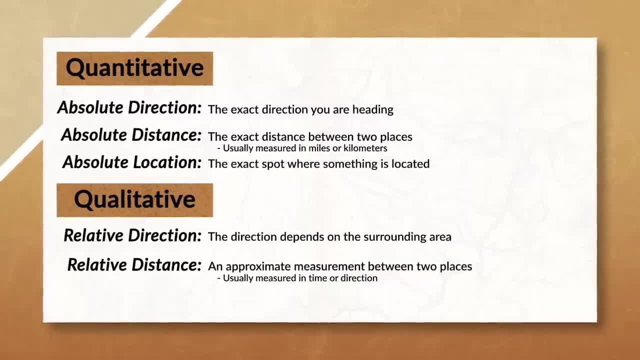 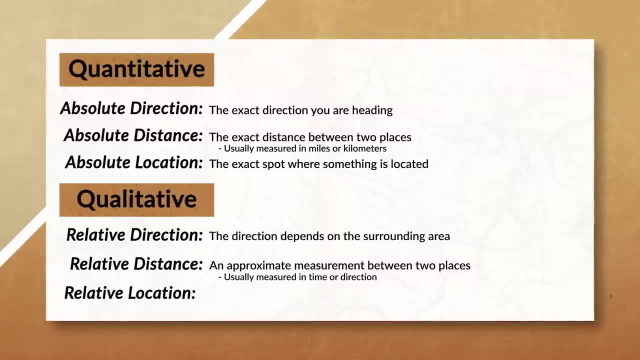 the Xcel Energy Center. Absolute location is when you're heading north of your current location. Absolute location is the exact spot where something is located, For example the GPS coordinates of a place. Here you are using longitude and latitude. Lastly, relative location is a description of a location using the surrounding geographic 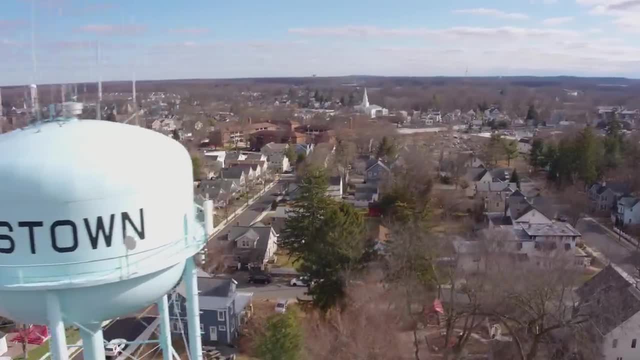 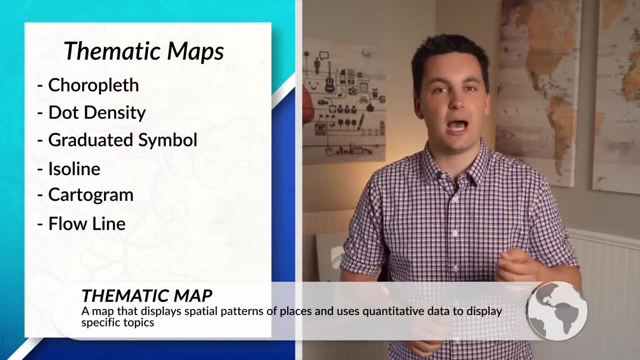 features. For example, my house is near the water tower and the fire station. Thematic maps, on the other hand, display spatial patterns of places and use quantitative data to display specific topics. These maps present the reader with specific information that can tell a story about an area. Chloropleth maps. 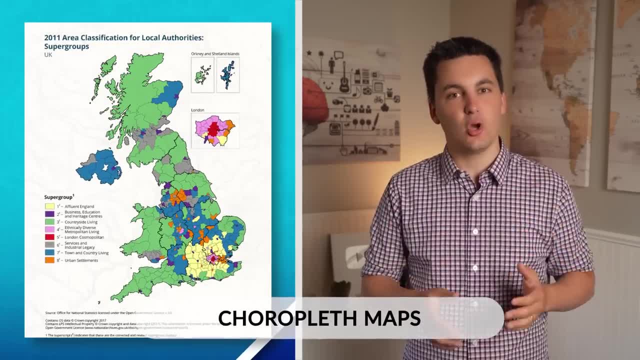 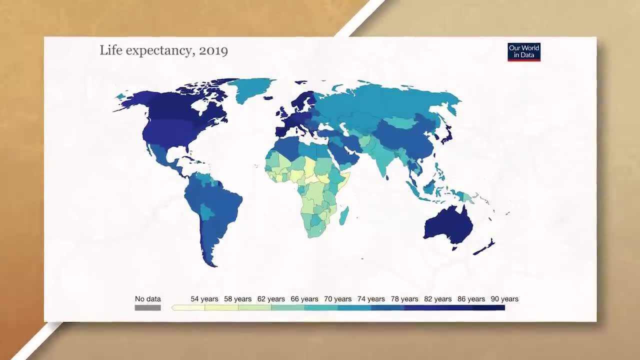 display data by using different colors. These maps are great at showing quantity and density, but use generalizations to display the information. For example, when looking at this Chloropleth map, we can see the average life expectancy for each country around the world. Notice that each color 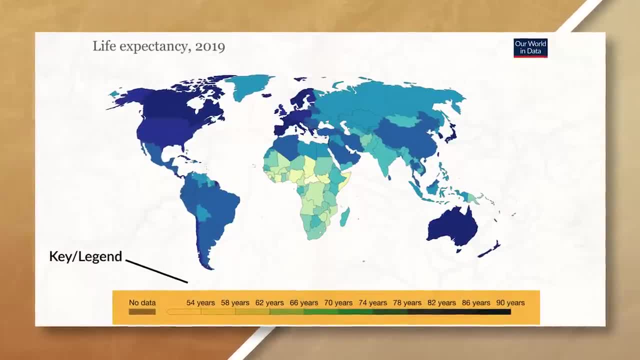 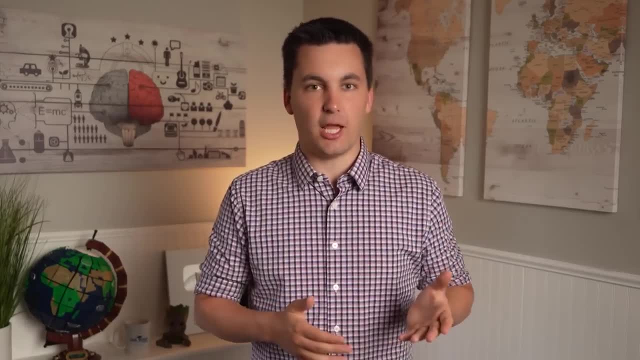 represents a different average life expectancy. The darker the color, the longer people in the country are living. One problem with this map is it's using generalizations to display the data. For example, take the United States. When looking at this map, we can see that the average life 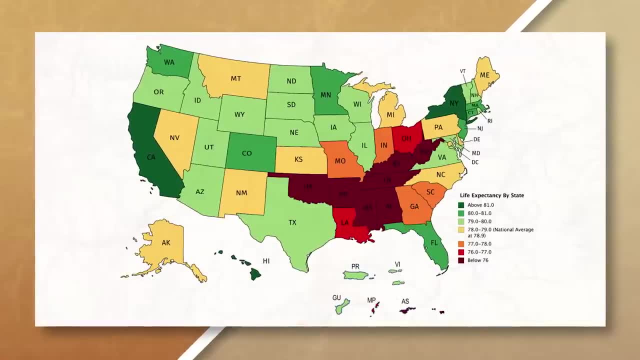 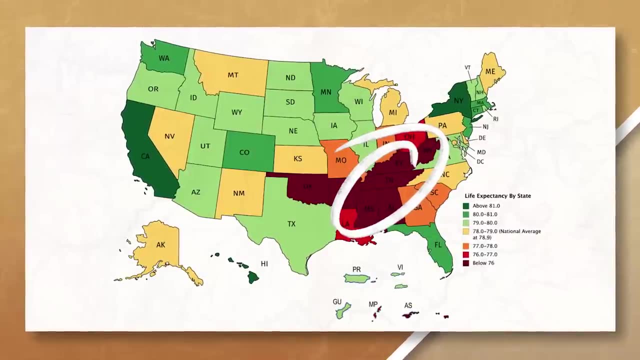 expectancy for each state in the United States is two years old, But if we change the scale of the map, we can see that each state in the United States has different average life expectancies, with some of the states having an average life expectancy well below the national average. 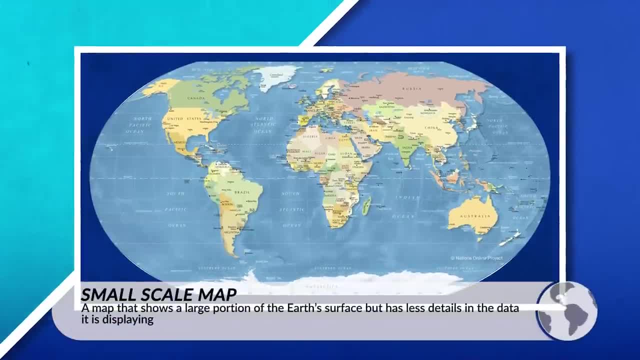 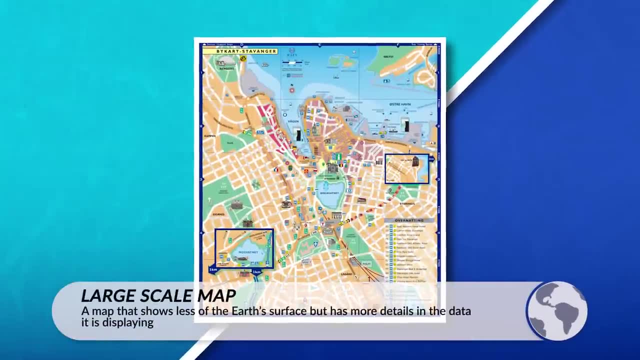 So here we can see the scale of the map was impacting our data and what we could perceive. Small-scale maps such as our global map have to use more generalities, since they're showing more of the Earth's surface, While large-scale maps, such as a map of a local community, 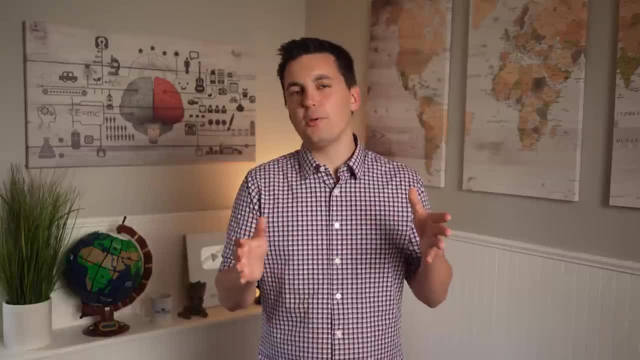 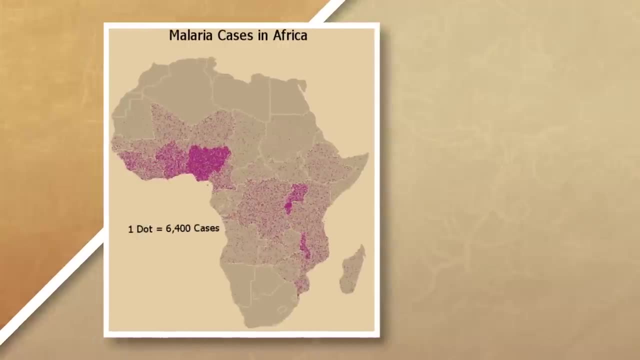 can use specific data and avoid generalities in the data. we want to be a little bit more specific with where the data on our thematic map is being displayed, So we don't want to use a chloropleth map. Well, we could use a dot density map. These 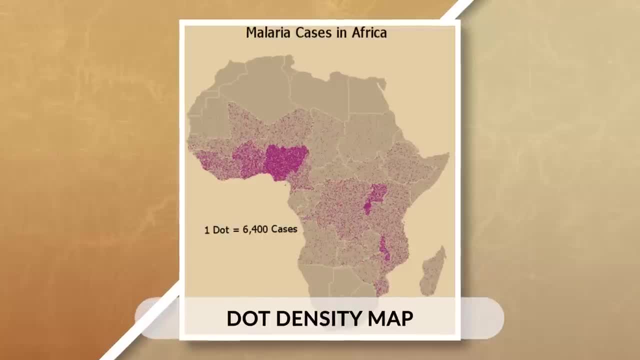 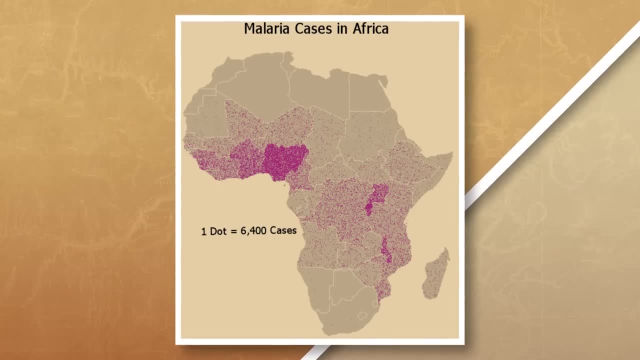 maps show data with points at the place the data is occurring. This allows us to see spatial distribution, but can become confusing if the data is clustered together in a specific area, If data, objects, items, people or information are close together. 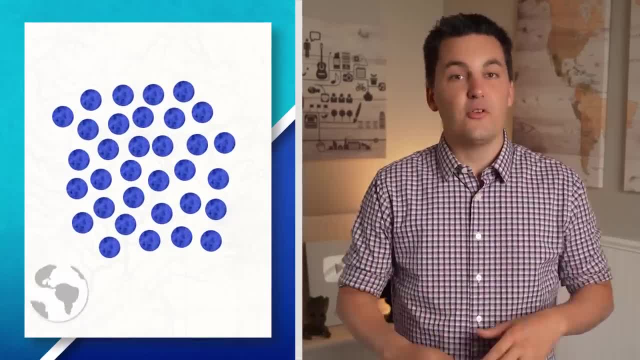 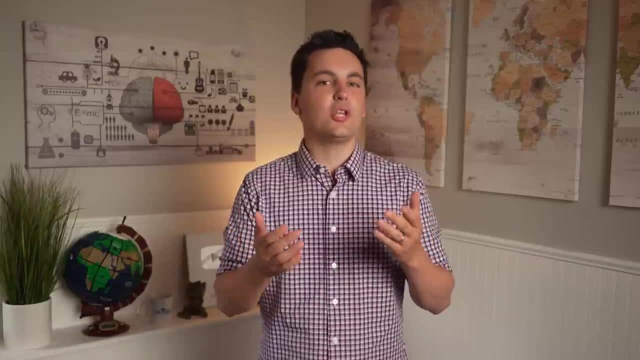 it means there's little space between them, So everything is packed together. If it is dispersed, it means it's spread out over a geographic area and there's more space between the items or information. For example, if we look at the racial dot map, which uses information from the United States, 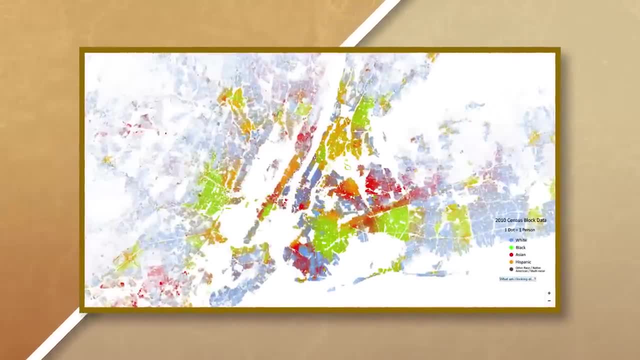 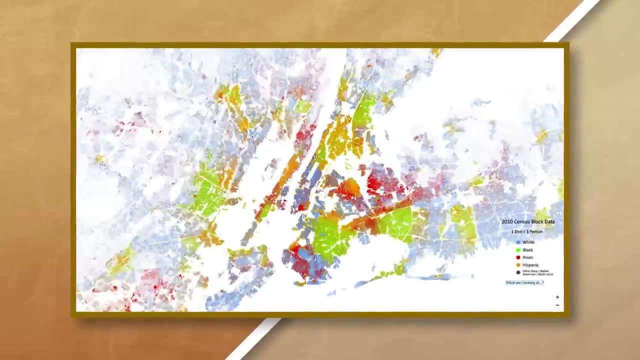 census, we can see where people are living in the United States based on their race. Each dot is one person. Notice, though, that in larger cities with a higher density, the dots seem to blend together as one, since people are living so close together, making it difficult to clearly see each dot. 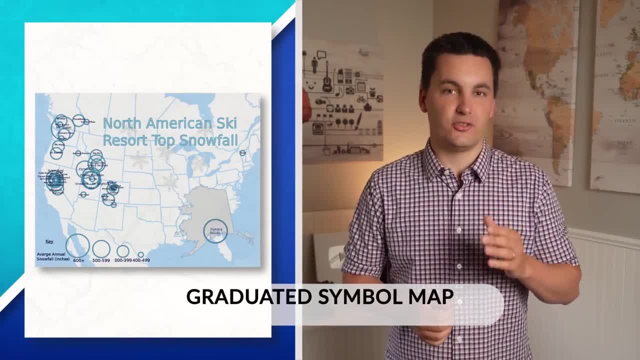 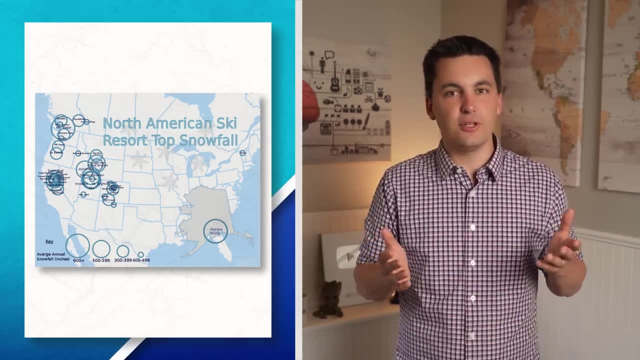 Another map that is similar to the dot density map is a graduated symbol map. These maps use shapes, items or symbols to show the location and amount of data. These maps are often really visual but can become confusing due to the overlapping information, For example, 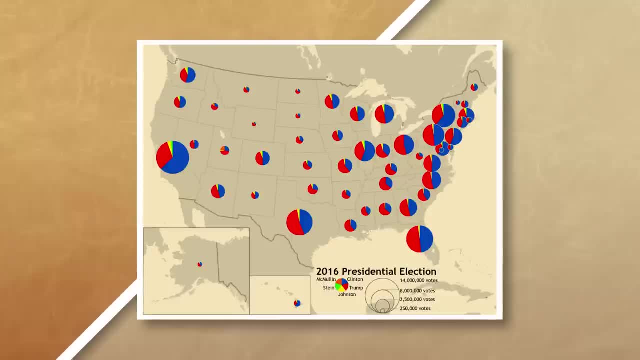 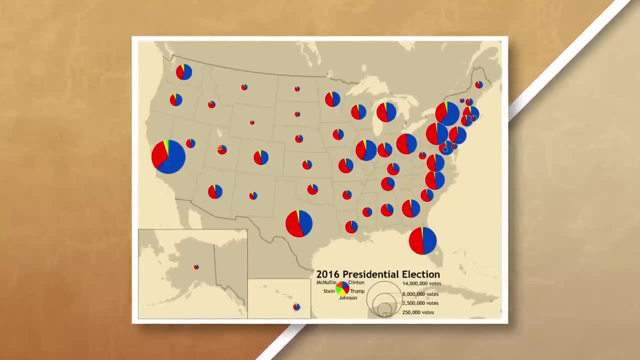 if we look at the 2016 United States presidential election, we can see. this graduated symbol map displays each state's voting breakdown and the amount of people that voted in each state. Iceline maps use lines to connect different areas that have similar or equal amounts of information. 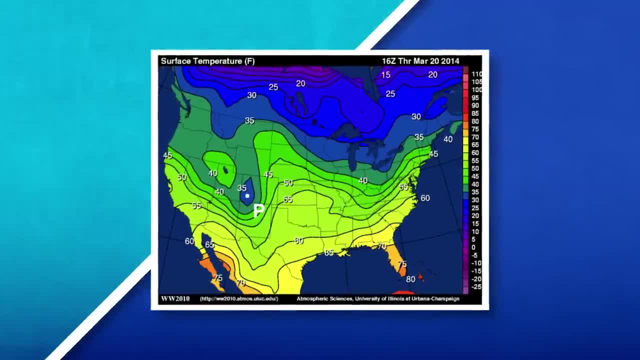 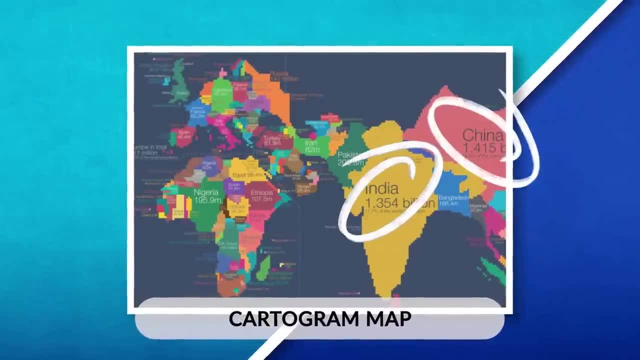 Oftentimes you'll see these maps as weather maps, but these maps can be difficult for people to read. Cartogram maps show data in a dynamic way, with the greatest value represented by the largest area. These maps are very visual and can clearly show differences. 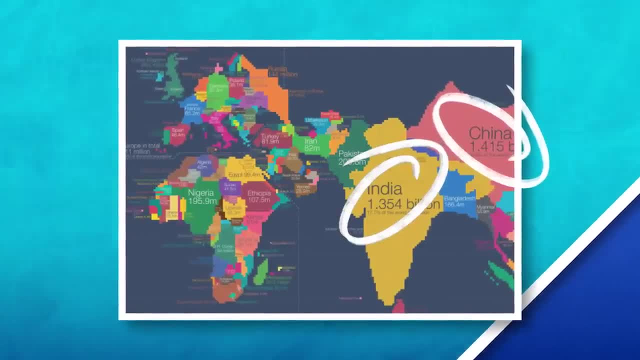 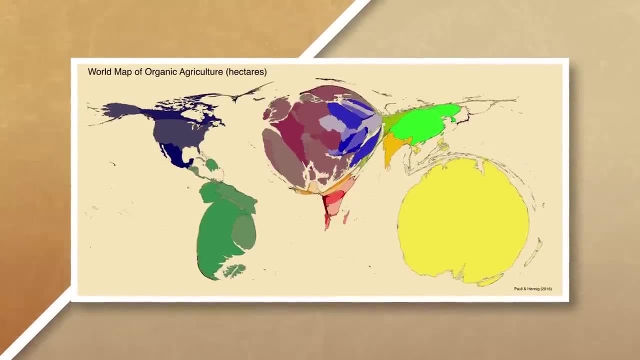 between different places, but can sometimes be confusing due to the amount of distortion of the shape and size of places, As you can see here. when looking at this cartogram showing organic agriculture, notice how some countries are almost non-existent on this map. 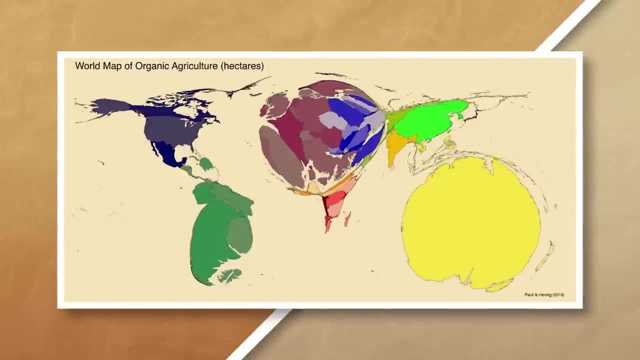 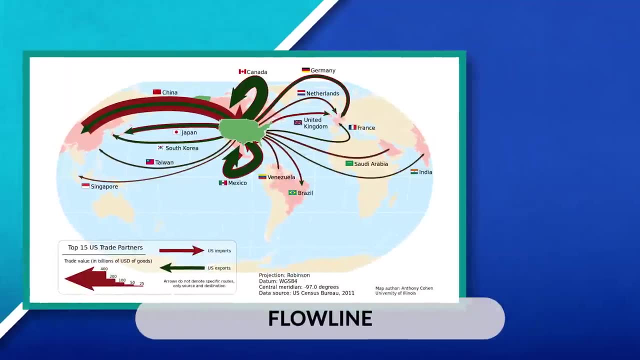 while others seem to dominate the entire map Here, the larger the country, the more organic agriculture is being practiced, and the smaller the country, the less. Lastly, there's a flowline map. These maps show the movement of different goods, people. 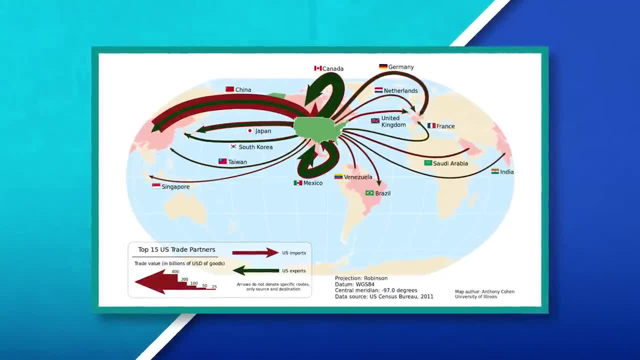 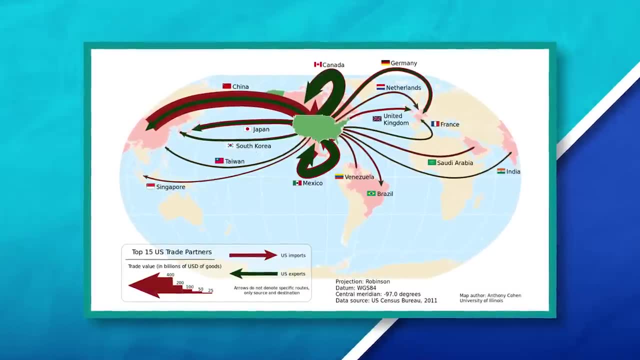 animals, services or ideas between different places, As we can see here when looking at the top 15 United States trade partners from 2011,. here we can see the amount of trade is illustrated by the size of the arrow and the direction of the trade is color-coded to show both exports.